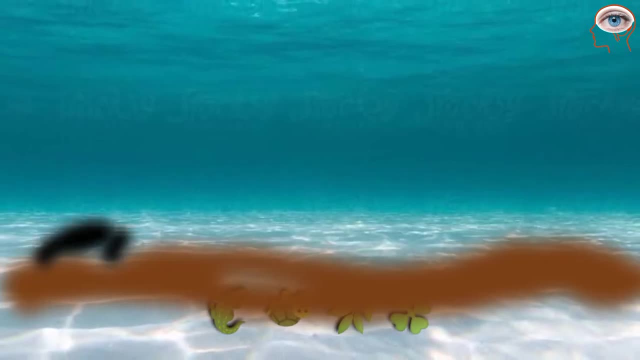 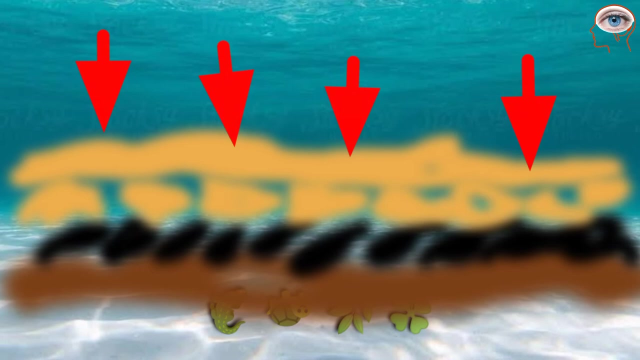 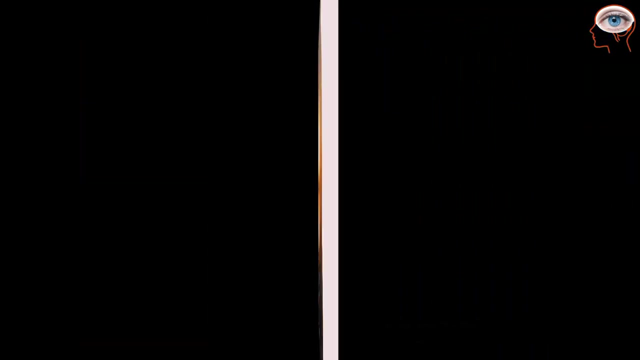 With the passage of time, it is further covered with shale and rock layers. Due to high temperature and huge pressure, it is converted into dark, viscous liquid that we call Petroleum, or also called the rock oil. Keep watching, keep learning with LifeSight. 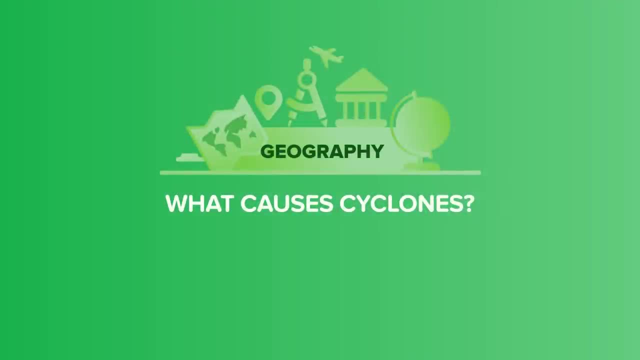 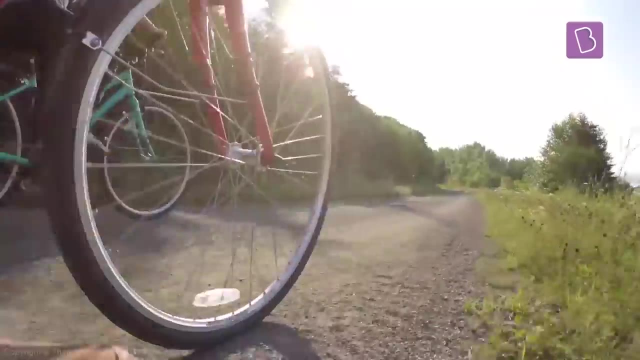 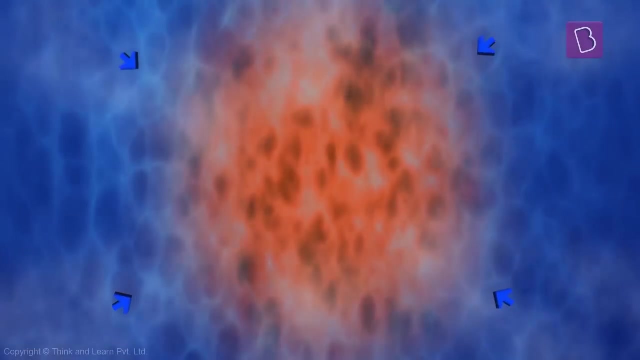 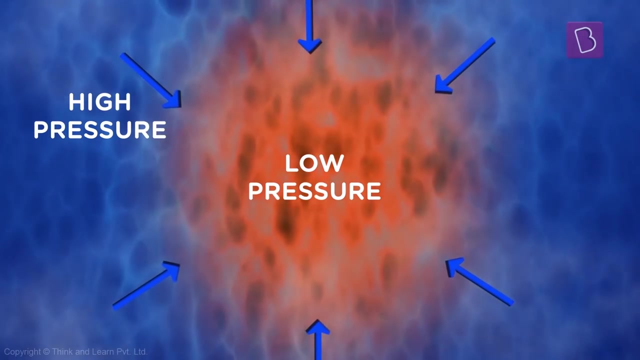 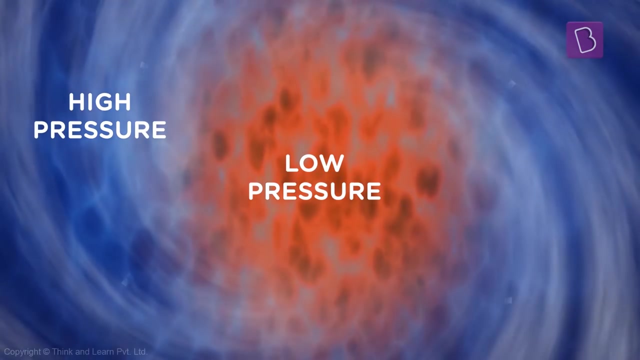 What comes to your mind when you hear the word cyclone? Well, I think about the wheels of a cycle or a bicycle. Now, sometimes, severe winds blow from a high pressure area to a low pressure area. When this happens, the winds start to spiral just like a wheel. These winds create disturbances in 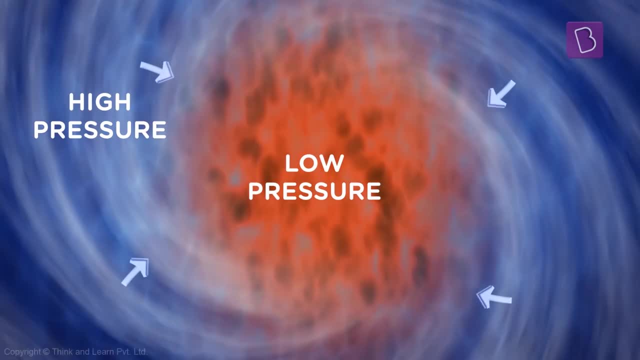 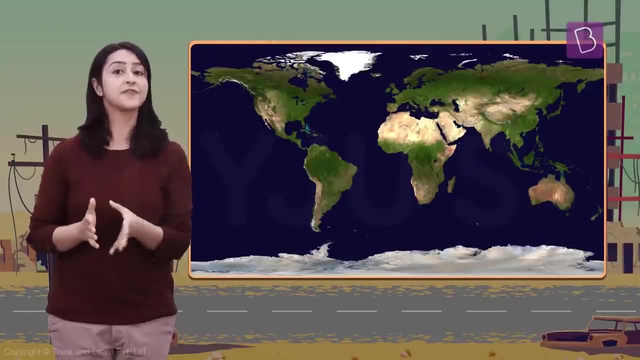 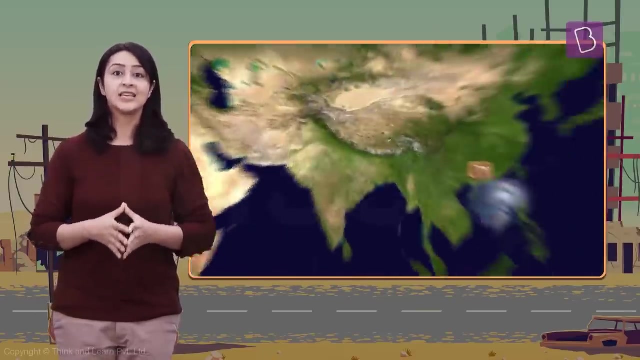 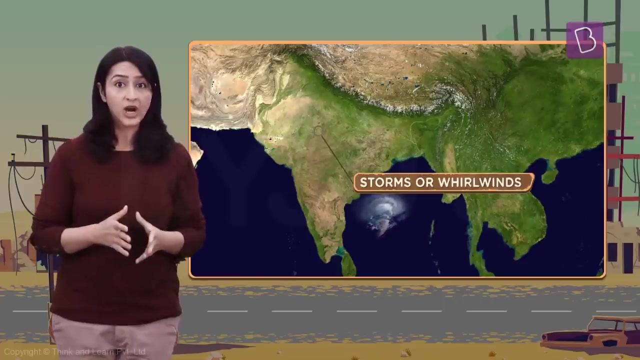 the atmosphere which results in heavy rainfall. This is known as a cyclone. Cyclones have different names in different regions. For example, they are called hurricanes in North America, typhoons in Southeast Asia and storms or whirlwinds in India. Most of the cyclones originate from 5. 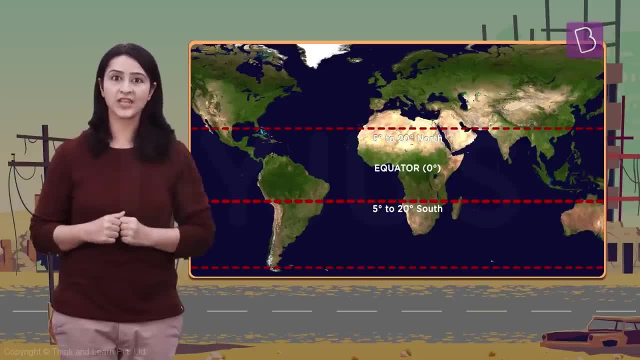 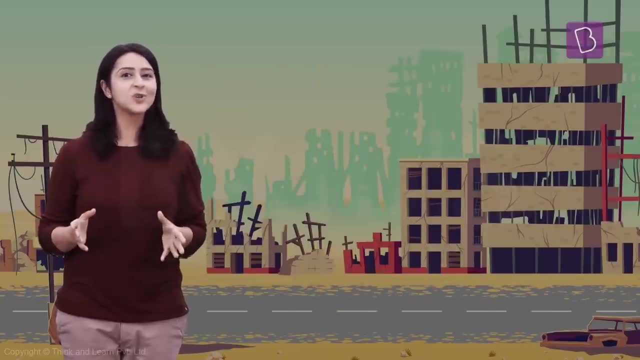 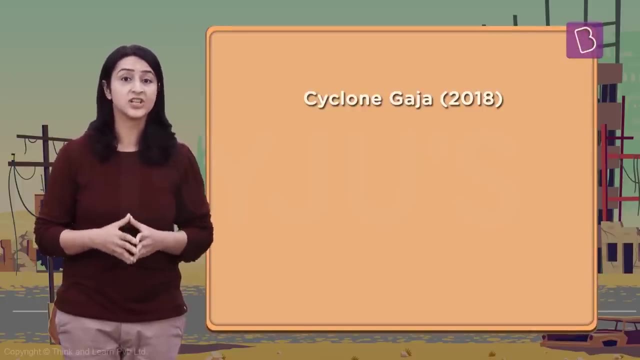 degrees to 20 degrees north and south of the equator. Because of this, they are called the tropical cyclones. I'm sure you would have heard of some common cyclones, such as Cyclone Gaja that occurred in 2000.. Cyclone Gaja is one of the most common cyclones in the world. Cyclone Gaja is 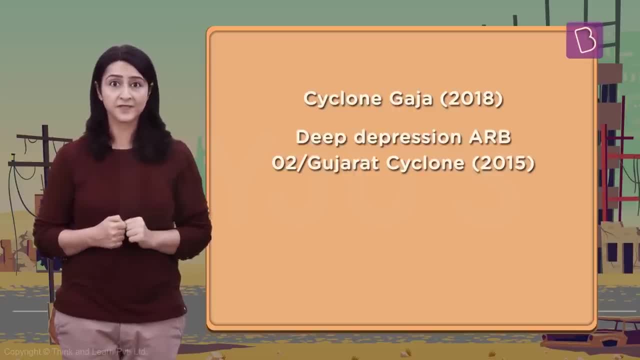 theenned, one of the most common cyclones in the world, one of the most rectified in 2018.. The 2015 Gujarat cyclone, also known as the deep depression ARB 2.. Then there are other cyclones, like cyclone Thane, cyclone Mora, and so on. Indiaoverukan. 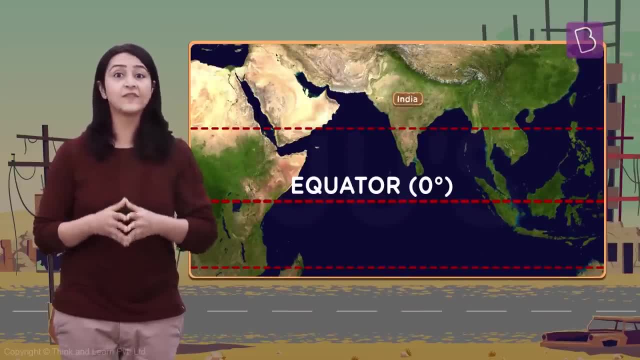 India is also highly vulnerable to cyclones. Well, this is because India is close to the equator falling in the tropical region. It falls from 5 degrees east toiph in пишpas and it's surrounded by thunder and lightning. When high vidéo becomes a phenomenon in in descendants's